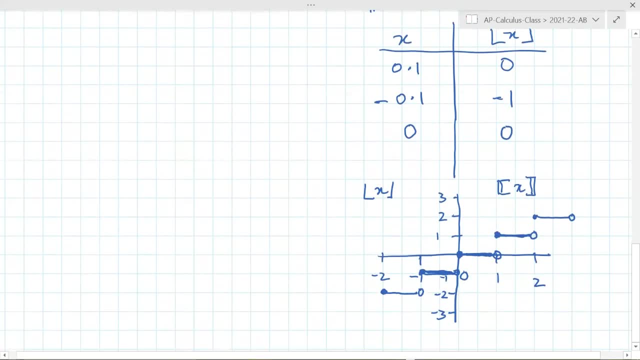 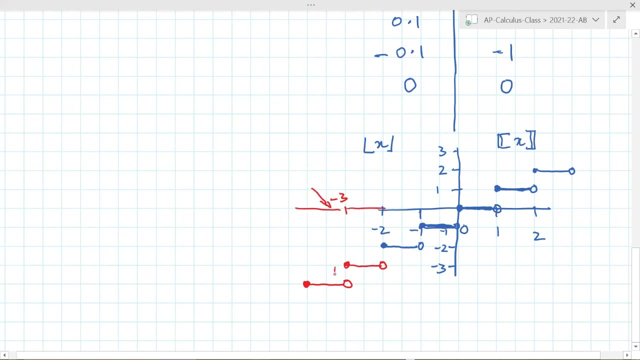 left of negative 3.. That means so we are just left of negative 3.. So we are here somewhere right Because we are doing negative 3 from the left. The minus on top of the negative 3 indicates that 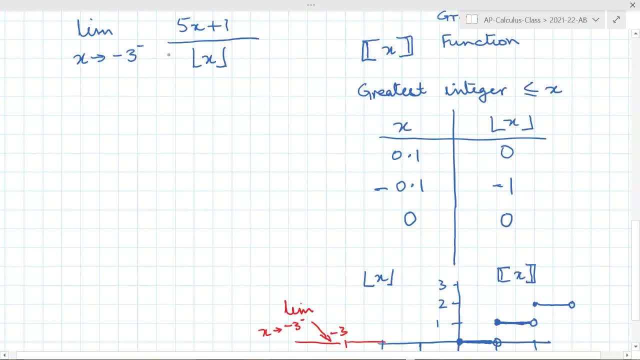 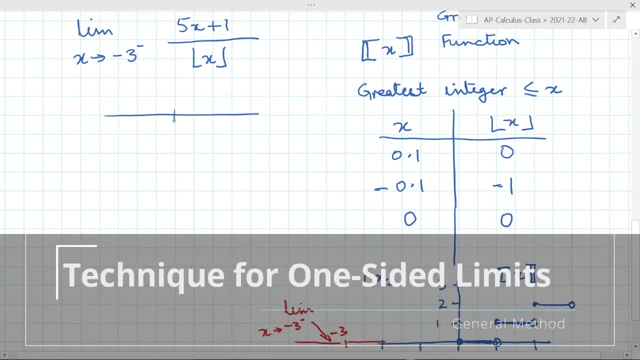 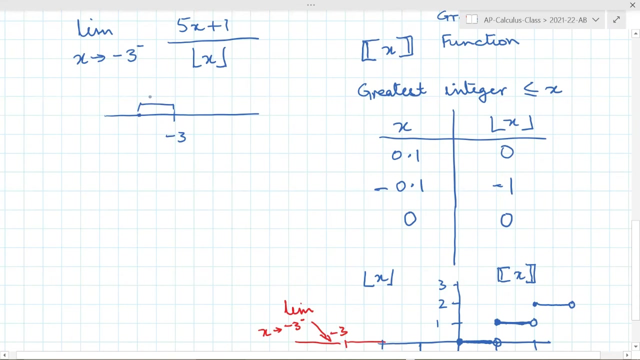 we are coming towards negative 3 from the left. So when you are trying to find one-sided limits, you can use this technique. This is negative 3.. Now I am somewhere here, right? So suppose this separation is t. t is a positive number. 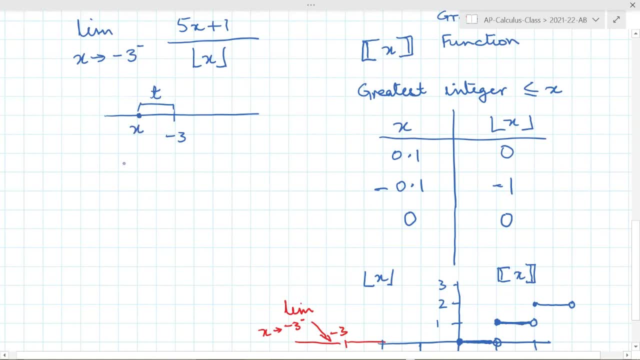 And this is my x. So what can I say? what is x? x equals. what is the relationship between x, t and negative 3? What's the relationship here? 3 plus 2 equals 5, right Here I have. 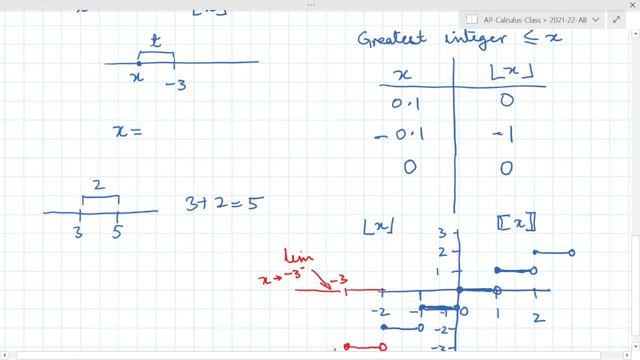 x, t and negative 3.. I have negative 5.. What is my x? It is maybe like x minus negative 3.. To put it simply, It is a negative 3.. I am negative 3, right, I am negative x plus negative 3.. I am negative x. I am negative x minus. 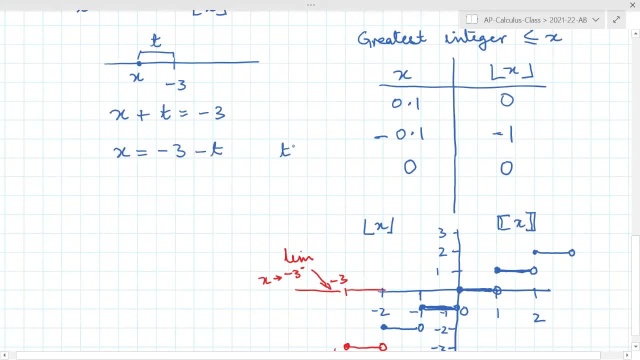 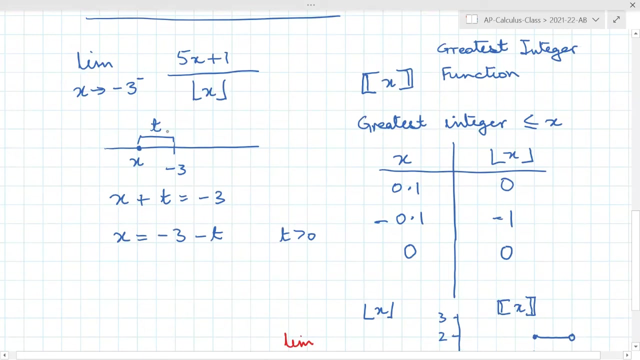 3. So what is x then? Where t is some positive number? right, Because only then x will be on the left. If t is negative, then x will come to the right, correct? So since we are trying to find a left-sided limit, we are saying, okay, x is negative, 3 minus t. where t is some positive. 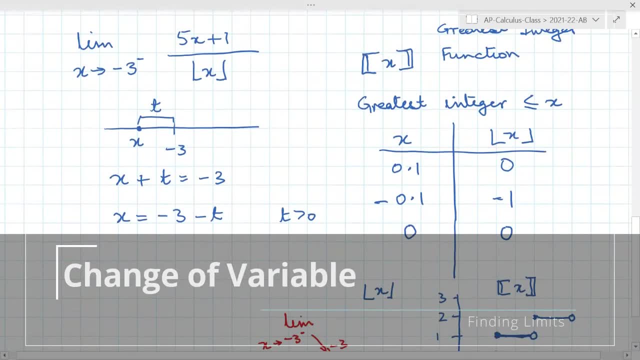 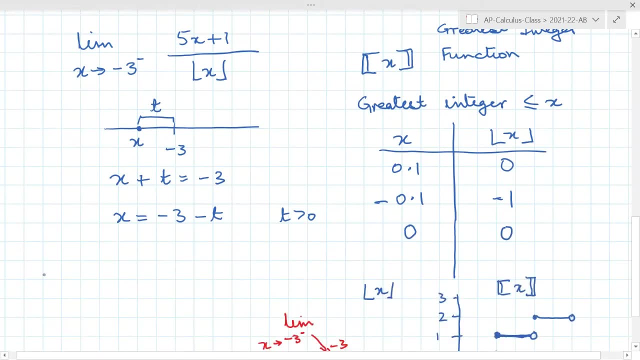 number. If that's the case, I can rewrite this limit in terms of t. I can replace x with negative 3 minus t. So limit 5 times negative 3 minus t. I'm replacing x with that Plus 1 over. 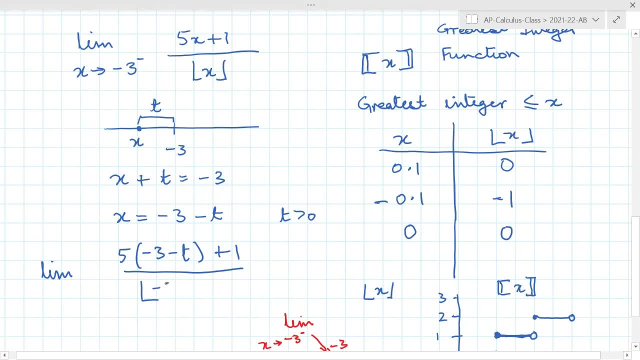 the greatest integer, negative 3 minus t. And as x gets close to negative t, what will t get close to? If x gets close to negative 3, means x is coming here, right? What is happening to t 0. See, t is becoming smaller, right? Only then x can come here. 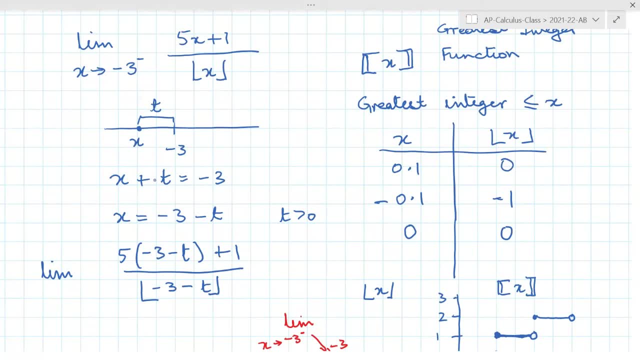 If t becomes bigger, then x will go away here. If t becomes smaller, then x comes close to negative 3.. And we are saying x is coming close to negative 3.. So what is happening to t? T is becoming close to 0.. 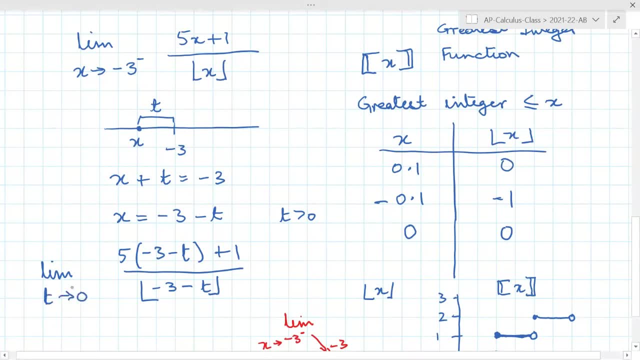 So T is going to zero. I have to find what to write here, right, Because I got rid of the X. Now everything is in terms of T, So I have to write the limit in terms of T, Because X was going close to negative three. 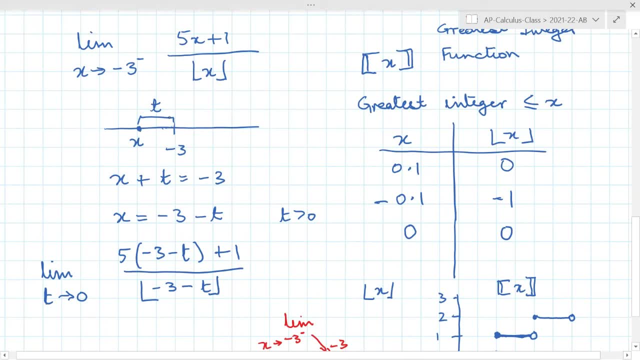 That means X is getting here and here and here. That means T is becoming smaller and smaller. So T is becoming close to zero. T is positive, T is greater than zero, But it is becoming smaller and closer and closer to zero. That's the only way for X to come close to negative. three right: 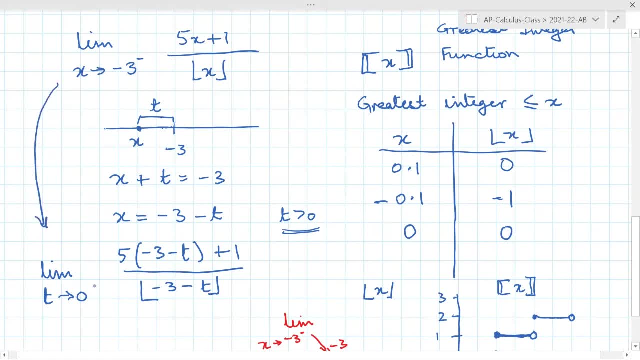 So I rewrote this limit like this: And now there is no left hand, right hand in this. right Now we can do the normal limit. So this is a way to replace a one-sided limit in terms of a normal limit. It is still one-sided, but we change the variables. 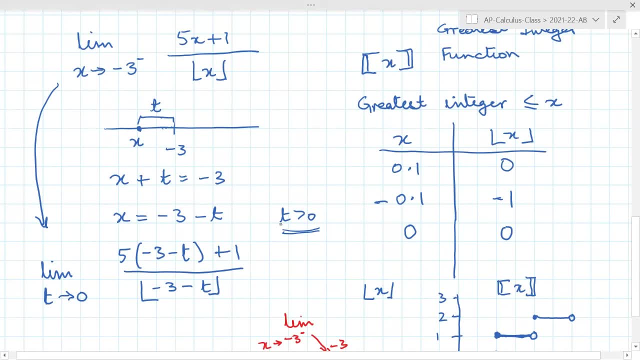 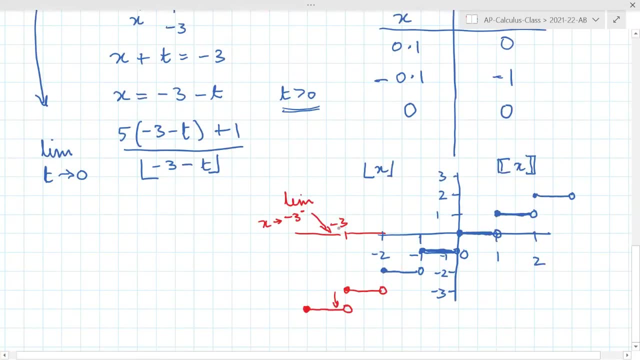 So it's not written as one side. We know T T is greater than zero And I can just write it like this. We still have to solve it, But I've just shown you the first step. We are over to the left of negative three. 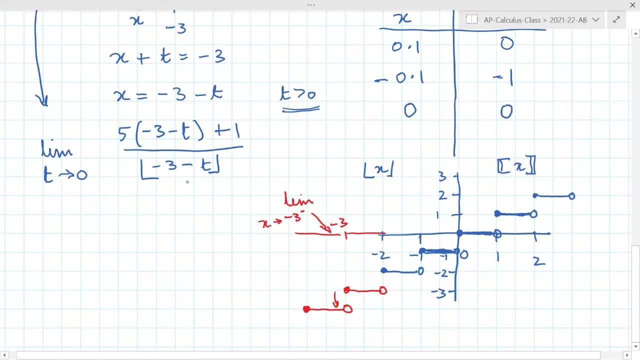 And we will stay on the left of negative three, because we never become equal to negative three. X never becomes equal to negative three. T never becomes equal to zero. That means we are operating here. We will be using this graph for X. So what is this value? 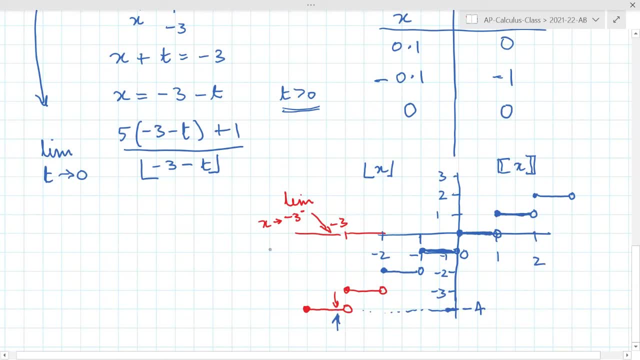 Negative four Because we are here. this greatest integer, less than or equal to negative three minus T, means we are here, So this value is negative four. You have to be careful here, because if you plugged in zero, then it becomes negative three right. 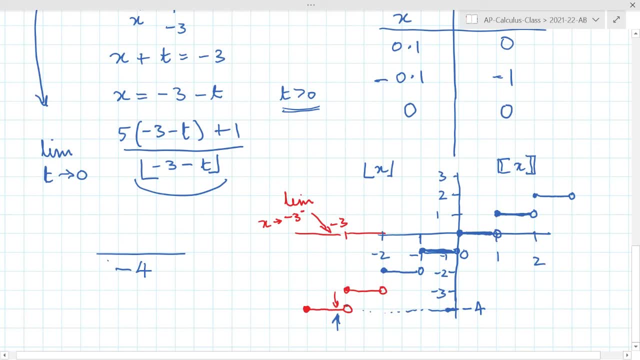 Then it will jump over here. We are not there. We are on the left of negative three. And here it is straight, Simple stuff. There is no greatest integer or anything like that. So here we can plug in zero. What do we get? 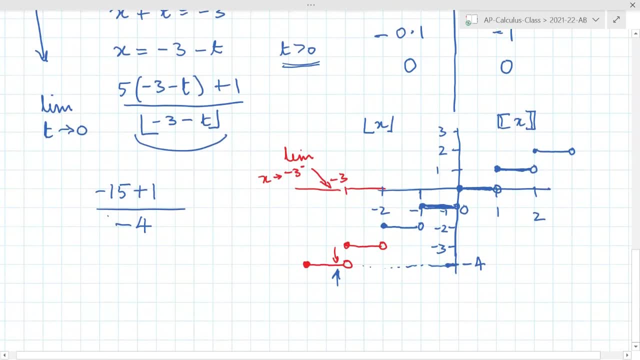 Negative 15 plus one, What is that? equal to Negative 14 over negative four, which is seven over two. That is the limit. We have to be very careful here, because there's a discontinuity here, right? Because if we plug in, T equals zero.